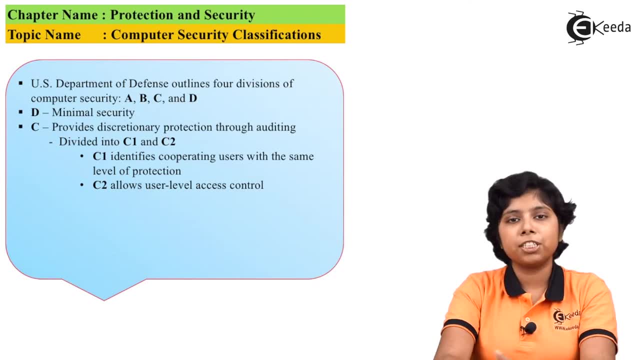 base, or pcb. all through our classification of this computer security, we will mention this tcb as a security measure protection. so this tcb is containing this user's access information, such as storing the passwords associated with each user. whenever the user is given input its original user id and password, this user has to give this privacy information. 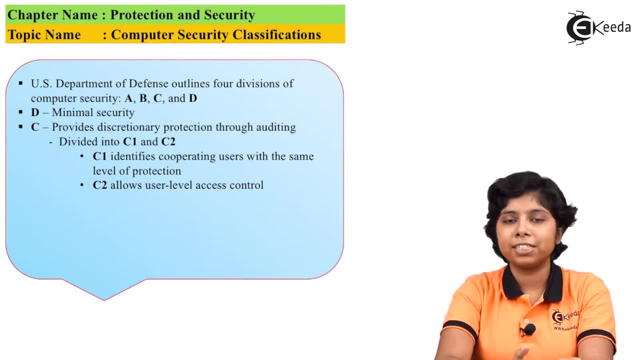 to the user. so this pn is responsible for this privacy security. so the user can see password is then match the password stored in this TCB to get the user authenticated for that access of file. Now this TCB is more authenticated when it is used in conjunction with any of the 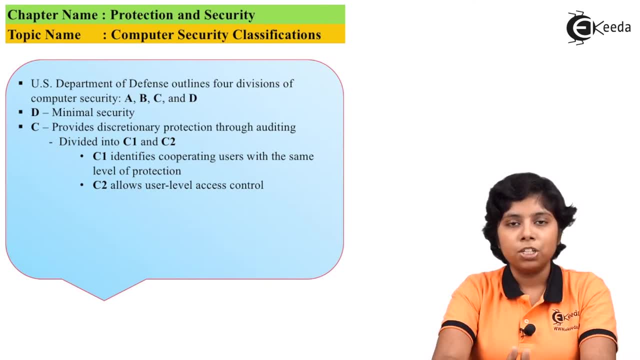 security measures that we have already described. So the class C1 can provide a basic security environment for the user authentication. Now the other class of this class C is the class C2.. The C2 gives, after the individual, access rights to this user authentication. it gives the individual 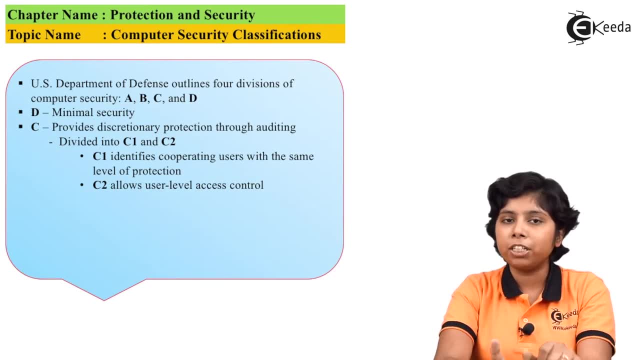 access rights to the files. So even if between the user some part of the user is given, only the access rights, say for the file read and some access to the file write, So the user identification is also divided into access rights to the files. that is known as this C1 on C2 classification. 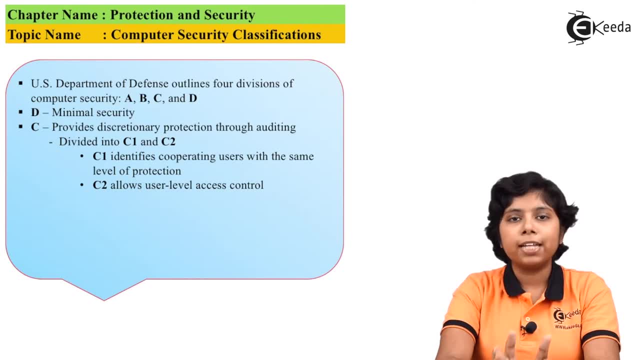 So the C2 provides more finer grain classification, That is, the access rights to the files and the devices, access rights depending on the user authentication only. So if the user is authenticated by class C1, then only it is considered to gain an access control on the access for files rights. So after C2 has been modified then it can gain a. 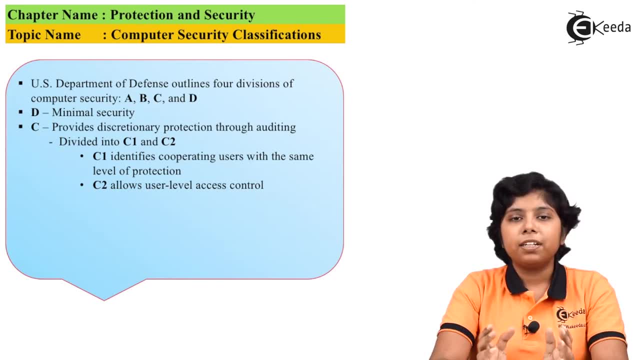 control or a particular mode of access inside that file. Now the class C2 also used to be secure, the more user authentication, password information along with a lock of this standard object, Say. for if the standard object is locked for a particular user, it then cannot be used by any other user in the system. So after the standard 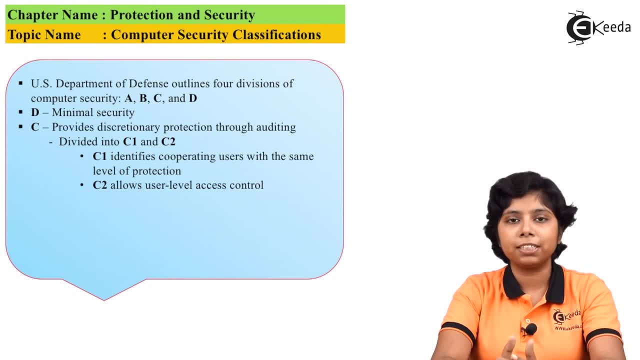 object is released by the particular user and is back to the system. now any user can get unlock of this object and access that particular object in use. Now we move to our next classification, that is class B. Now class B have three parts, that is b1, b2, b3. now b1 is more like the system implementation of the c2, which has 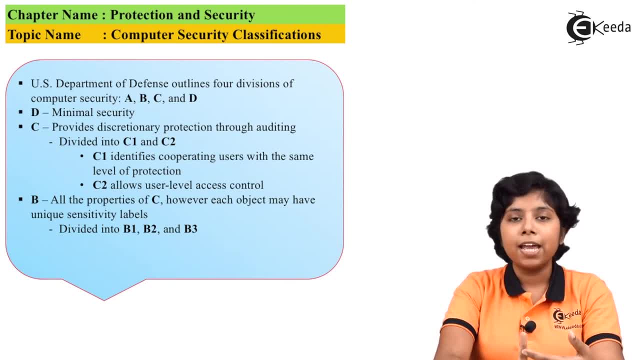 have user authentication as well as the file access rights, and it also has an sensitivity level attached with each of these access rights to the files. this sensitivity level will choose us among that which control to be given to which file, say for a user, which is given control of an. 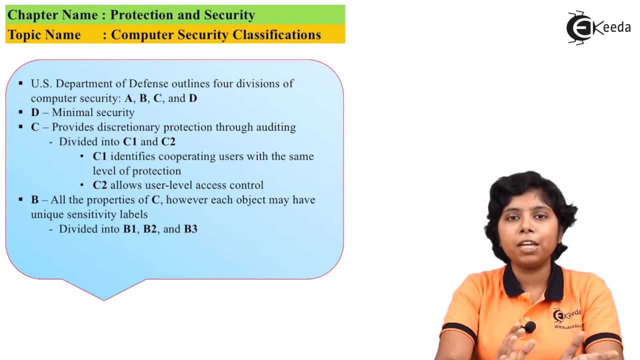 confidentiality information access will cannot be given control of an top level secrecy of the particular information. so if the top level secrecy is mentioned then the user cannot begin control of the confidentiality information. so it is gone upwards like this: first the user is gained on a normal file, then confidentiality, then top level secrecy. so like this the sensitivity level is: 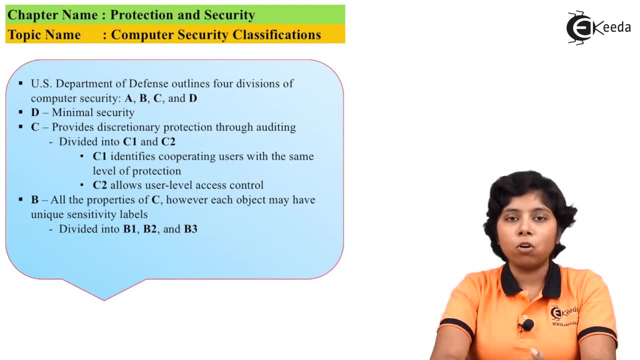 attached with every access right through the files and after the confidentiality information access access right is given to the user to the file And also other than this user authentication and password. these B1 levels also provide some finer gain control by providing access to the two level user identification. 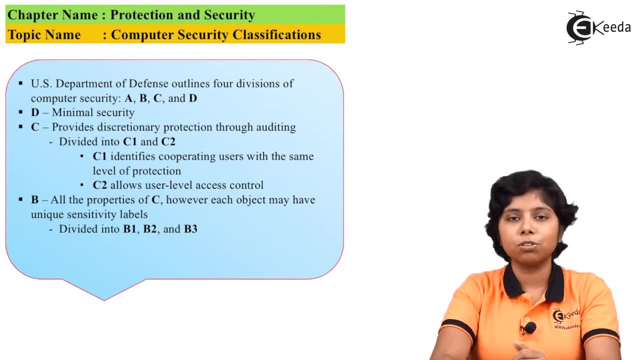 That is, whenever a higher control can have the access to the lower control organization, but not the vice versa. Say, for an user which has an access over the top secrecy level, information rights can have the access to confidentiality rights, but the vice cannot be done. 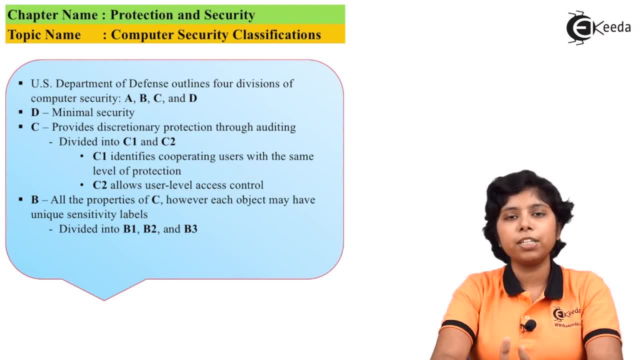 So in this way, B1 provides an user authentication with a sensitivity level access to it. Here the TCB is more designed accurately to give us the more information about the access control list that is used to maintain that which user will be used which access control and then granting and denying the 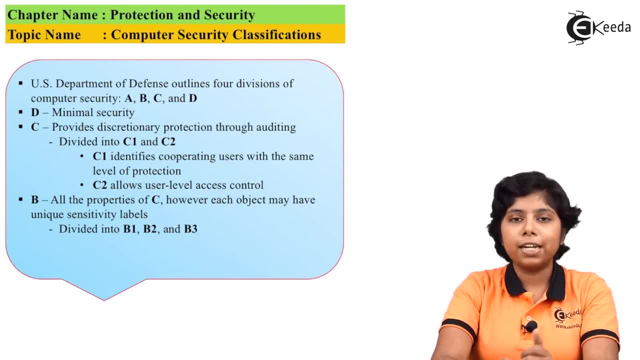 access on that access control list basis. The next type of the class that B provides is B2.. Now B2 provides all the facilities of B1, along with the facility that it provides the security measures that is considered at the network level, So when the data is generally considered transfer. 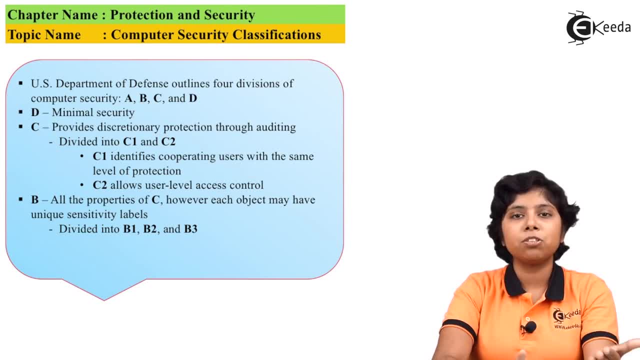 among this network level. so the security that is applicable to the networking scheme or say via the networking medium, is achieved via this B2 level of security. Now it also specifies the resources uses, like the maximum and minimum policy or the privileges that is attached to a resource, So a network, information and a remote computer.